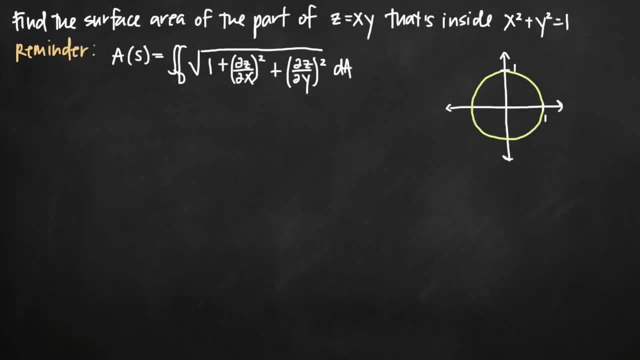 Today we're going to talk about how to use double integrals to find the surface area of the part of this function- z equals xy- that lies inside x squared plus y squared equals one. So, as a reminder, here I have the formula for surface area using a double integral. 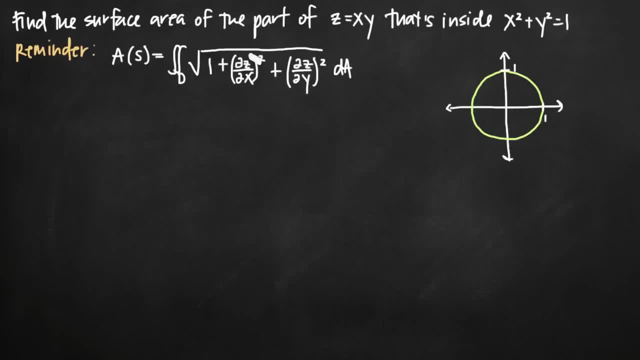 Notice that the only thing real complicated about it is just that we have to take partial derivatives of z with respect to both x and y. So we can go ahead and do that now, Because we're finding surface area of this function, z equals xy. we want to take partial derivatives. 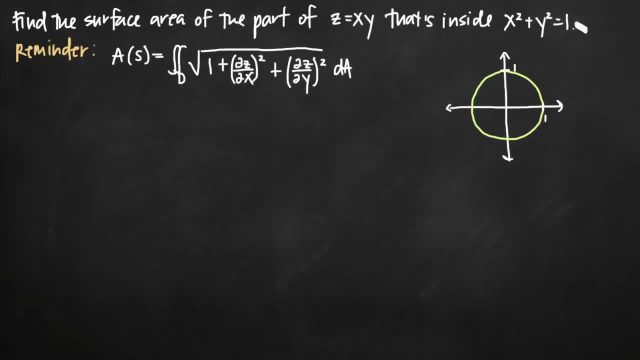 of this one. We're going to use this equation- x squared plus y squared equals one- to find the bounds, our limits of integration, because this equation here is bounded by this one. We're looking for surface area of this that lies inside this, So let's go ahead and take. 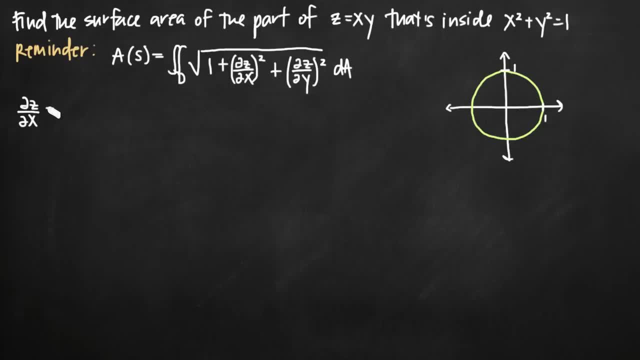 partial derivatives of our function, z with respect to x and with respect to y. So we're going to do that. When we do that, remember, if we take the partial derivative with respect to x, we treat x as the variable and y as the constant, which means that in this case, 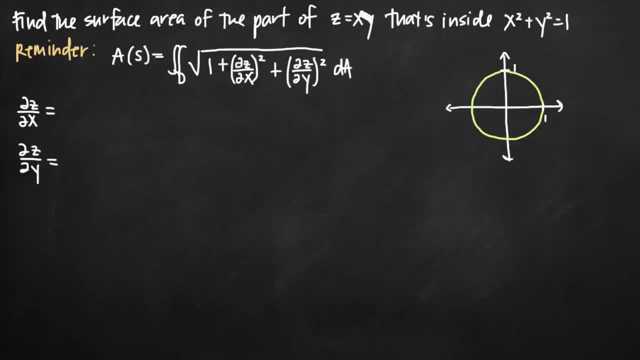 y is just a constant coefficient on this first degree x variable here. so the partial derivative with respect to x will just be y. The partial derivative of z with respect to y will just be the opposite scenario and we'll end up here with x. Now we can plug both of those. 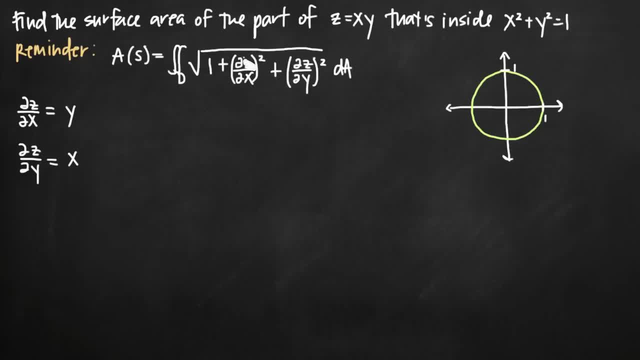 in to our double integral here in place of these partial derivatives. So what we're going to do is we're going to take the partial derivatives here Now. all we need is upper and lower limits of integration for both x and y Now, because we just have this circle here, right? 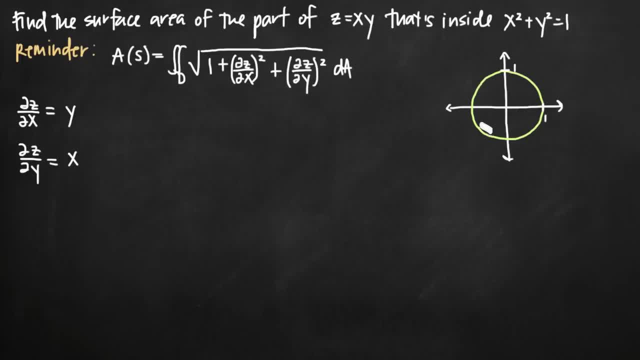 x squared plus y squared equals one. the graph of that is just the unit circle where the radius here is one out of distance of one from the origin. so here's our graph. we can treat this as a type one region, And if we're treating it as a type one region, we can go. 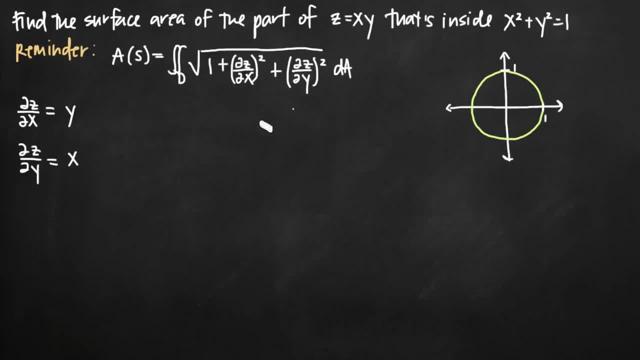 ahead and integrate, first with respect to y and then with respect to x. So we're going to do that. So our surface area integral- here double integral, we'll say the surface area is going to be equal to. I'll leave placeholders for our limits of integration and we'll go. 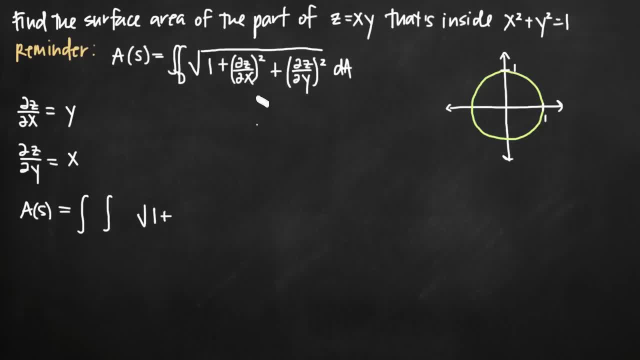 ahead and write everything else in. So we have one plus the partial derivative with respect to x, which we know is just y- We're going to square that and we're going to get y squared. And the partial derivative of z with respect to y, we know is x When we square. 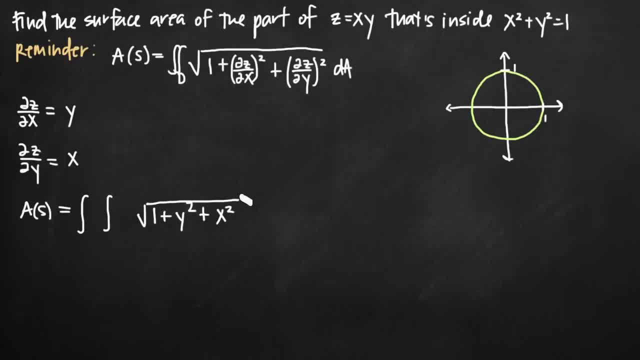 it we get x squared And then dA. here we're going to replace dA with dy dx, and the reason is because we can treat this as a type one region. We can draw vertical cross sections here that would allow us to find the area of this region here. So we'll integrate first with respect to y and 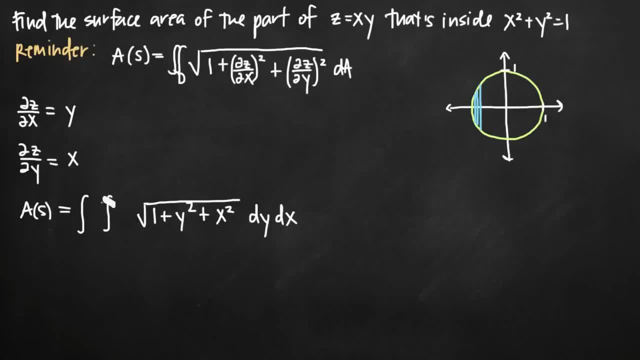 then with respect to x, because we can treat it as type one. That means that our inner integral here is going to have to have limits of integration with respect to y, because the dy is on the inside. Since dx is on the outside, our outer integral will have limits of integration with respect. 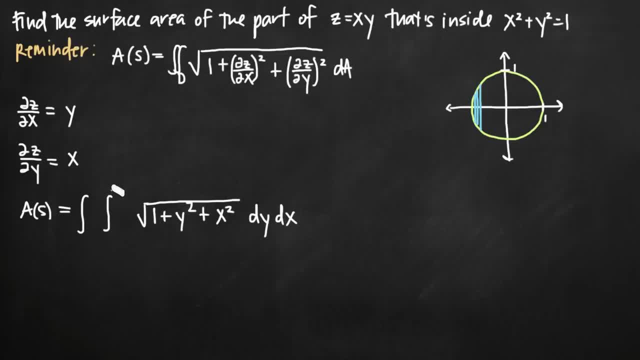 to x. So, because dy is on the inside, our limits of integration with respect to y need to be functions for y in terms of x, And the way that we'll do that is by solving our bounding equation here for y in terms of x. When we do that, we'll subtract x squared from both. 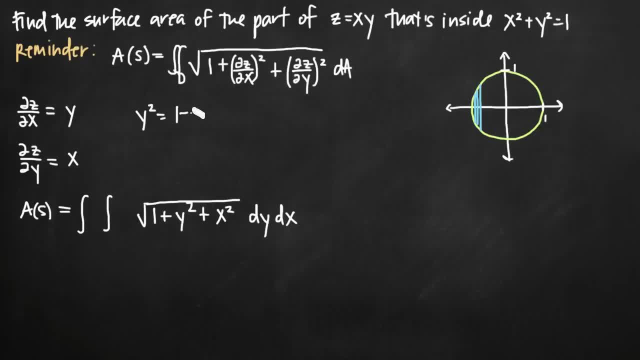 sides and we'll be left with y squared is equal to one minus x squared. So that's going we get: y is equal to positive or negative square root of one minus x squared. Therefore, we know that our upper and lower limits of integration for y are these two values here. 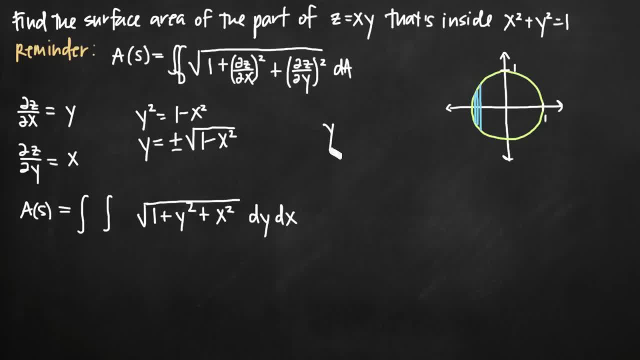 So we can say that y will be greater than or equal to negative square root of one minus x squared, and less than or equal to the square root of positive or positive square root of one minus x squared. Those are therefore going to be our negative square root of one minus. 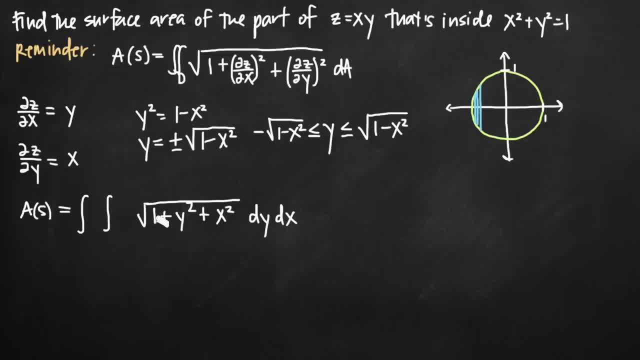 x squared and positive square root of one minus x squared. Now, because we're integrating first with respect to y, we said that our limits of integration with respect to y need to be functions of y in terms of x. Because we're integrating with respect to x. second, 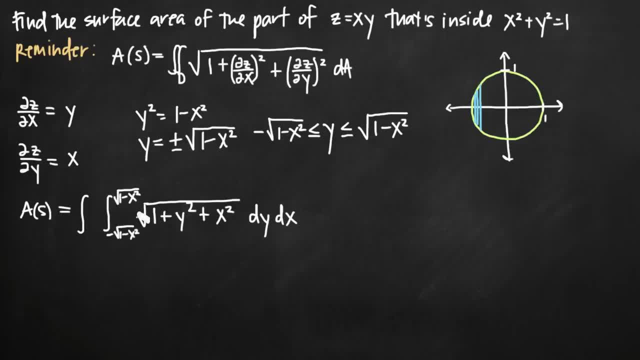 and dx. here is on the outside. our limits of integration with respect to x can just be constants. Well, the first thing we're going to do is integrate the limits of integration with respect to x. So we're going to integrate the limits of integration with respect to. 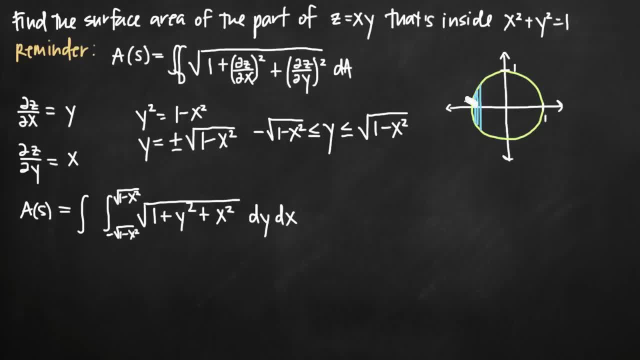 y, As we can see from our circle here, the leftmost value that x can possibly attain is right here, and that's: at x equals negative one. The rightmost value that x can possibly attain is right here: at x equals one. So negative one to positive one are our limits of integration. 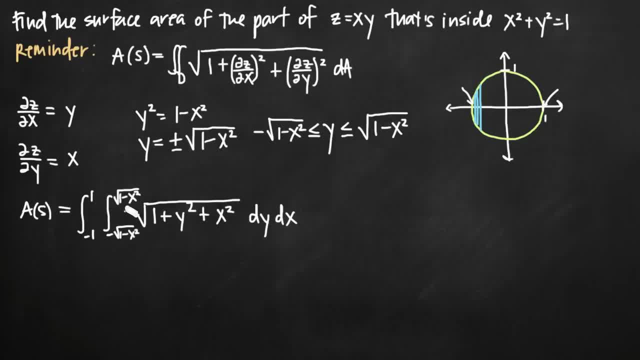 for x. Now we've got our integral set up and we just need to solve it. The easiest way to solve this integral, especially since we're dealing with a circle here, is to change the integral from correct to positive. So we're going to take the integral from the leftmost. 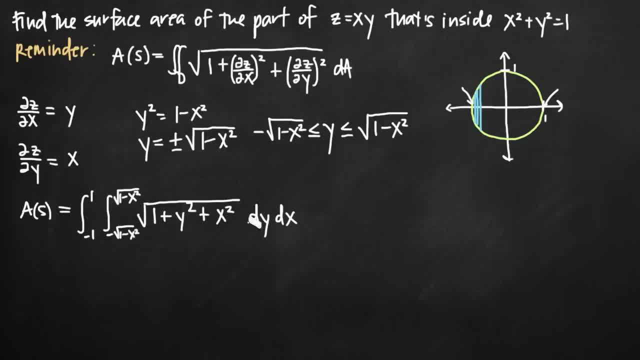 two sides of a circle, negative one and x equals negative one, And since we've got like 2 and in place that we're going to integrate negative one to positive one and then negative one will send us a product. This particular product will send us a Ой. each other plus both. 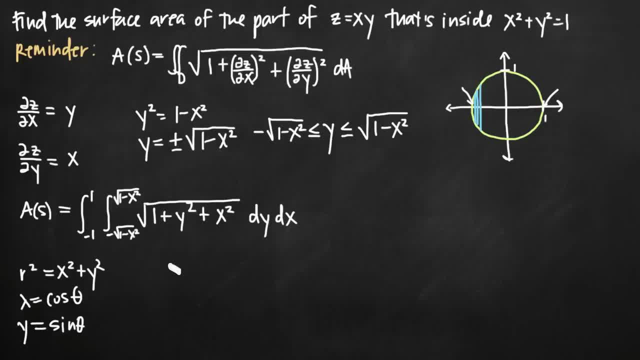 So that's right. negative one equals negative one plus positive one, which is negative one, equals the instructional aspect of directly. Squeeze the equation, So remove above the uh series of products. Look at equation four. I'm not just some placeholders for those, but remember that we have: r squared equals x squared plus y squared. 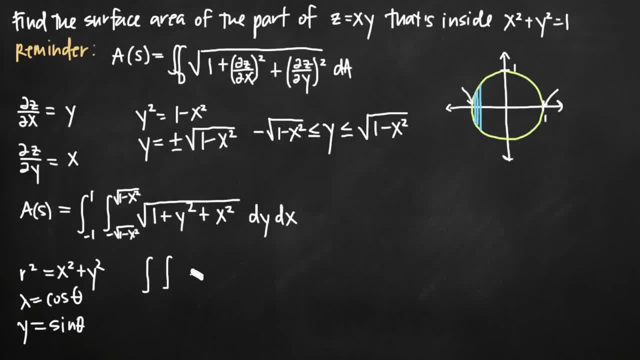 So inside of our integral we can go ahead and substitute r squared for x squared plus y squared, and you can start to see why it's very convenient for us to change to polar. So we get one plus r squared, putting r squared in place of this y squared plus x squared. 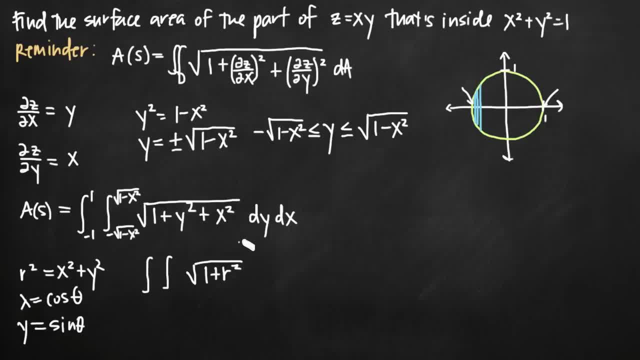 here. Then whenever we change to polar, dy dx always gets replaced by dy dx. dx always gets replaced with r dr d theta, in that order. if you have dy and then dx, We get r dr d theta. Now, because here we're integrating first with respect to r, because dr is on the inside. 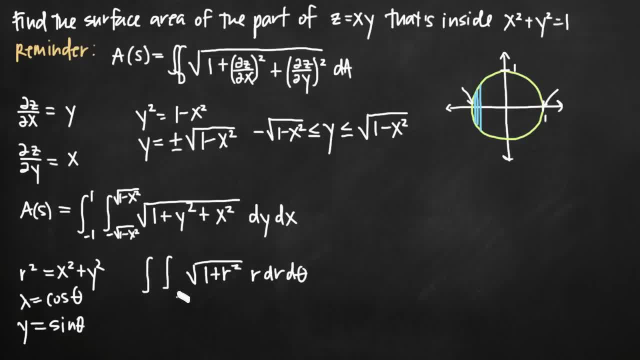 our inside integral here is going to need to have limits of integration with respect to r. Well, if we look here at our circle, our limits of integration with respect to r the lowest value that r can attain if we are treating this now as a integral. 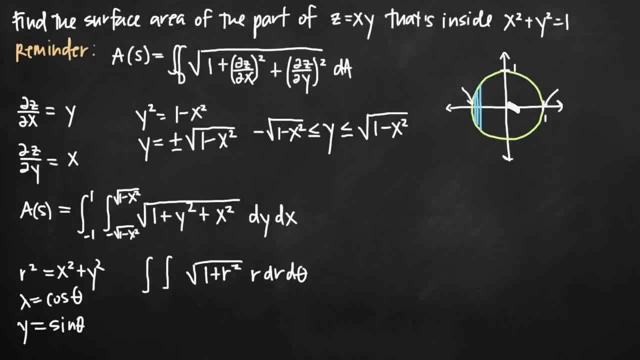 Polar coordinate plane. here The lowest value r can attain is zero, which is right here, at the origin right. So zero is our lower limit of integration. Our upper limit of integration is the largest radius that is attained anywhere inside this circle. So how far out does r go in any direction? 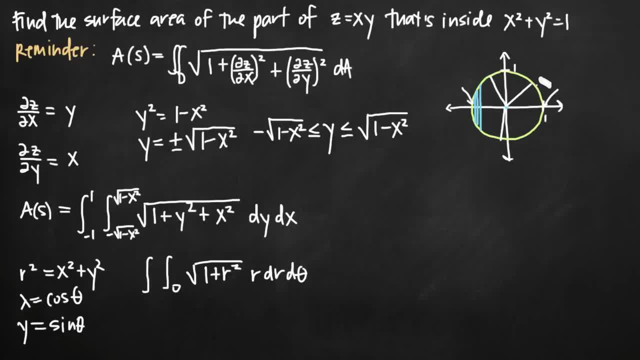 Well, in every direction that I go, the radius is one. So the largest value that r ever attains, the largest distance away from the origin, is one. Now, these are my limits of integration here with respect to r. I'm also going to need limits of integration here with respect to theta. 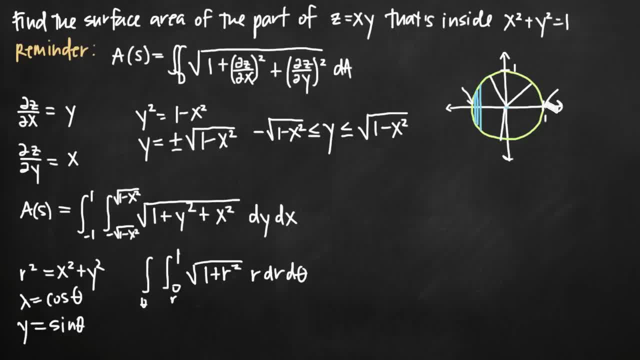 Now for theta. remember, theta is the angle. We want to talk about the smallest and largest angles that bound this circle. Well, since it's the entire circle and we want the whole area, obviously the smallest angle is just the angle zero here along this axis, and then we can go around the entire circle. 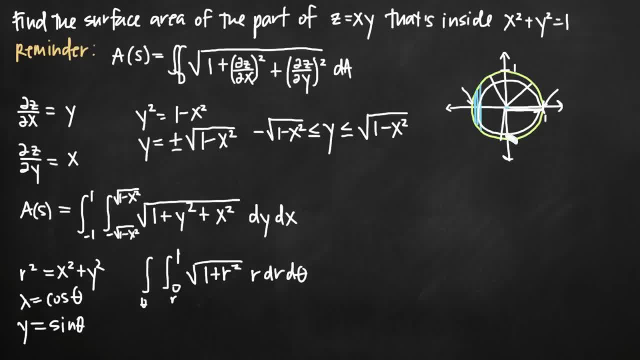 all the way back to an angle of two pi, because we want to get the full circle here. If we were just asked for the semicircle here above, let's say the x-axis, then we would want upper and lower limits of integration of zero to pi. 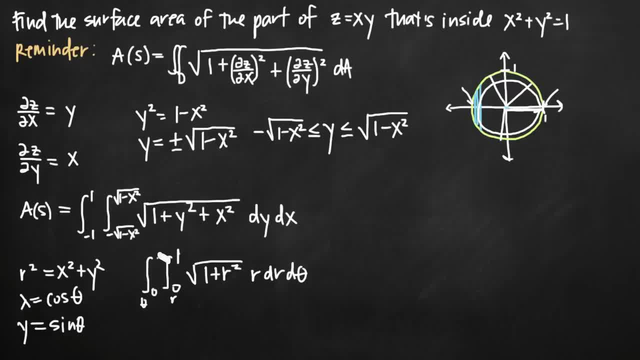 But because we want the entire circle here, we're going to say zero to two pi. Now, as you can see, changing from Cartesian to polar coordinates makes our integral look a lot simpler, so it's going to be easier to solve. The way that we're going to solve it is with u. 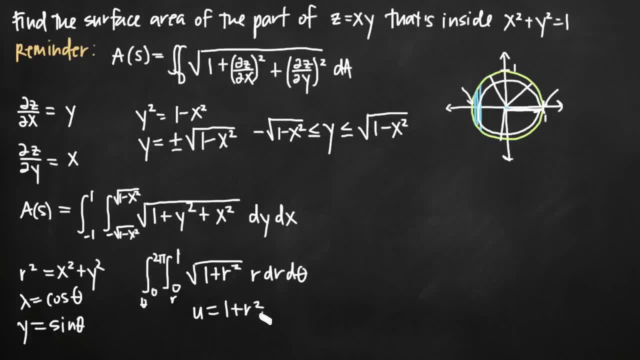 We'll set u equal to one plus r squared. We'll take the derivative of u and get du. The derivative of one plus r squared will just be two r and we add dr there. as always, We can solve this for dr by dividing both sides by two r and we see that dr is equal. 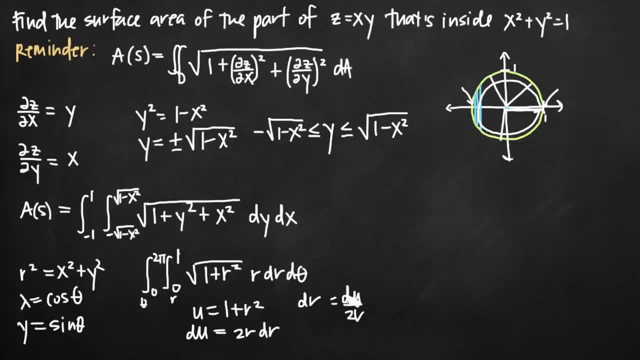 to du over two r. Now if we go ahead and make substitutions back into our integral, we'll get zero to two, pi of zero to one. So we get one of the square root of u times r. we can't forget this r here, and then for: 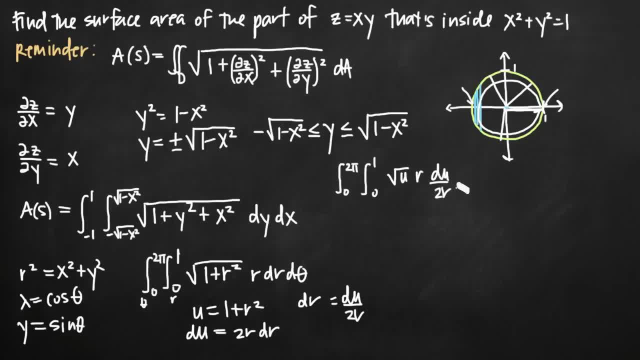 dr. we got du over two r and then we have d theta. Now notice, our r variables here are going to cancel and what we're left with is the integral from zero to two, pi of the integral from zero to one. This two here in the denominator can just get brought out in front as one half, and then 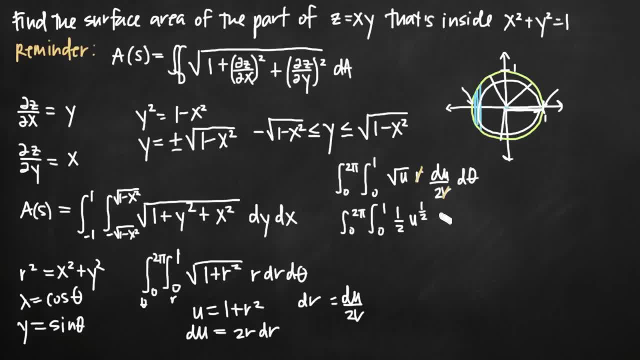 square root of u is the same as u to the one half power du squared. So we're going to solve this. So we're going to take our integral d theta Now, when we integrate here with respect to u, we'll get zero to two pi. 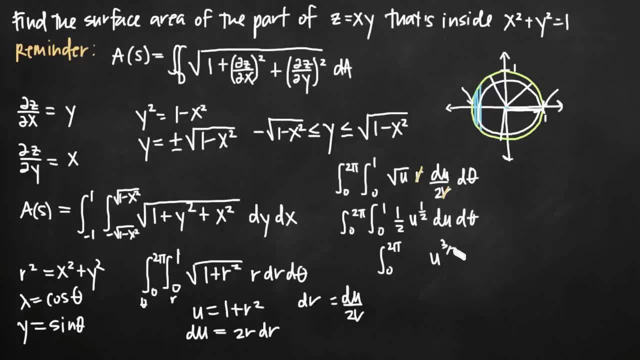 We'll add one to the exponent to get u to the three halves, We'll divide the coefficient by our new exponent. so one half divided by three halves is the same as one half times two thirds. So we're just going to end up with one third out in front here and then we're going to 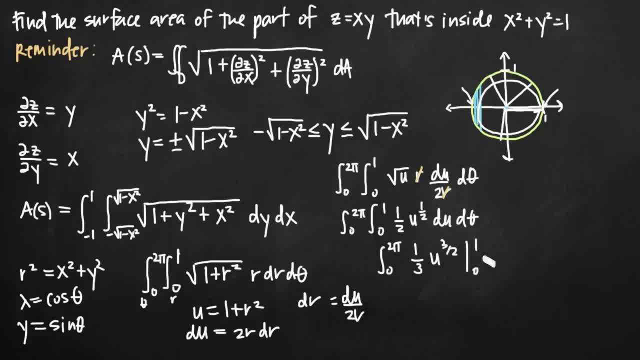 be evaluating that on zero to one after we back substitute for u. So we'll have d theta, We'll back substitute for u. Remember we said u is equal to one plus r squared, So zero to two pi of one third times one plus r squared, raised to the three halves power. 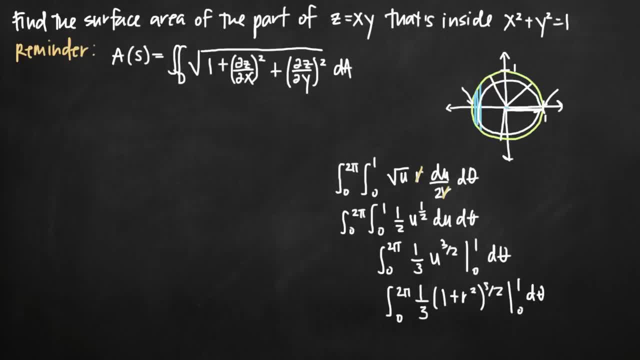 on the interval zero to one and of course d theta. Now, if we plug in our upper limit of integration, one to our one third times, one plus r squared raised to the three halves, we'll get one plus one. inside here, One squared is just one. 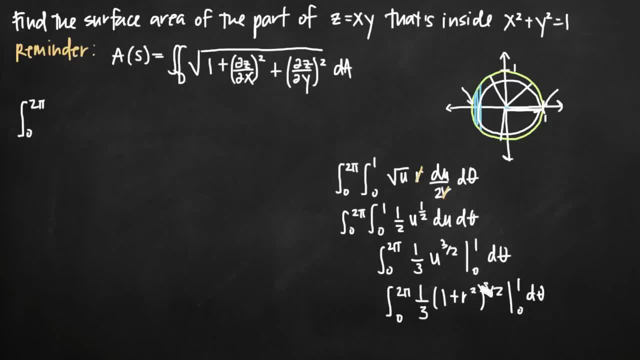 So we get one plus one, which is two. Two raised to the three halves is going to be square root of eight, because two to the third is eight and then eight to the one half, taking into account the two. here in our denominator, eight to the one half is square root of eight. 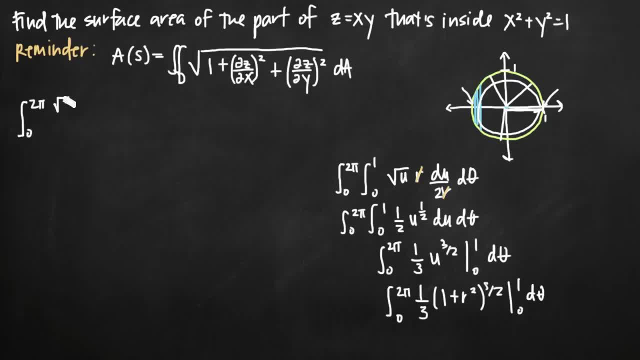 Square root of eight times one third is just going to be root. eight over three. when we plug in one, When we plug in zero, we'll get zero. squared here is zero. One plus zero is one. One raised to the three halves is still zero. 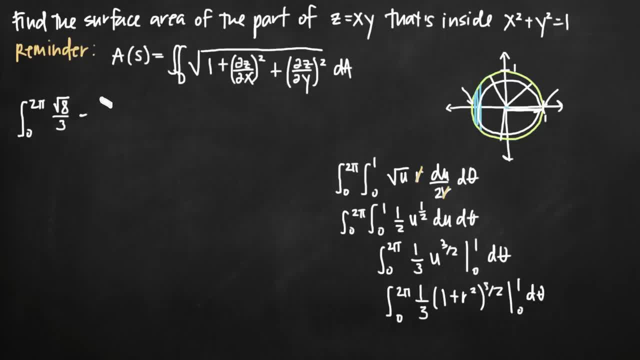 We'll just one times one third is just one third, So we get minus one third and then d theta. Now, if we integrate this with respect to theta, we'll of course get root eight over three times theta minus one third times theta, evaluated on the interval zero to two pi. 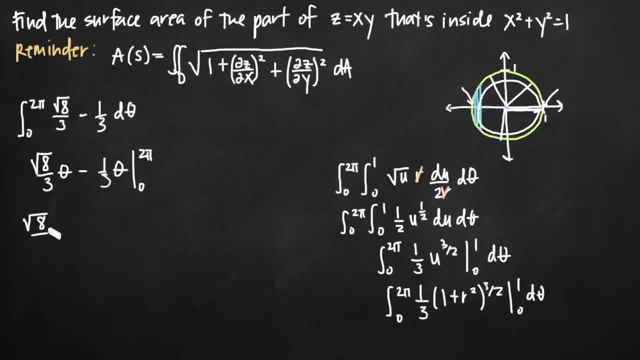